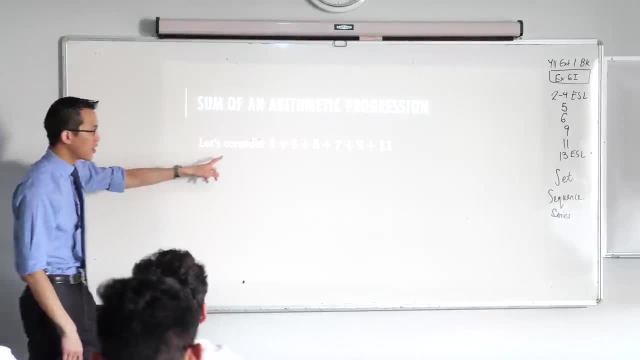 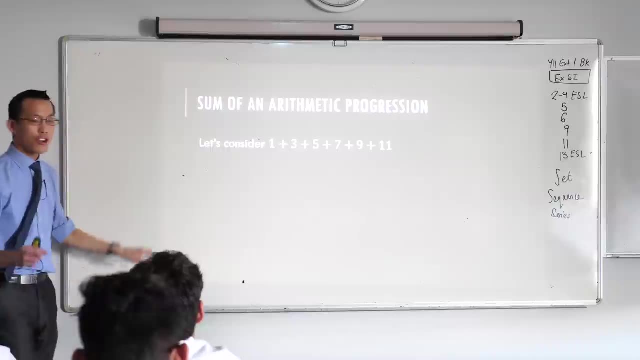 I know that it's sufficiently simple that we could just go and do this by hand, Like you: just add up 1 plus 3 is 4 plus 5 is 9, and then on and on and on. Right, I know you could do that, but what I want to do is try and. 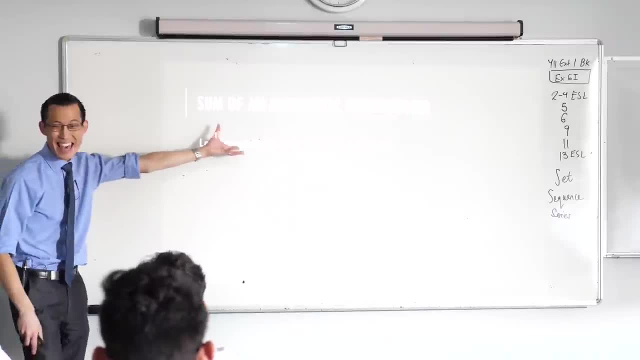 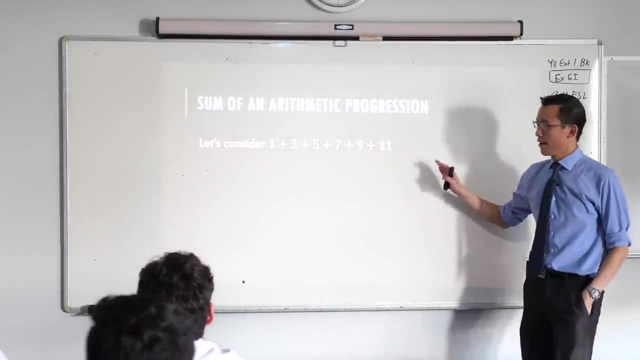 you know, analyze this for deeper structure. I want to see if we can understand this better so that when you do get a sequence or a series that's like gross and messy and you can't just do in your head, can we come up with a more systematic and simple way to do it? 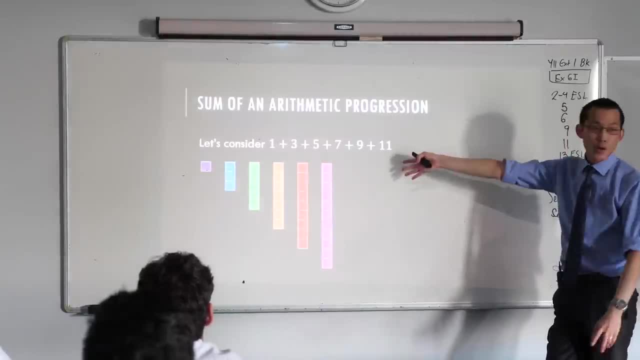 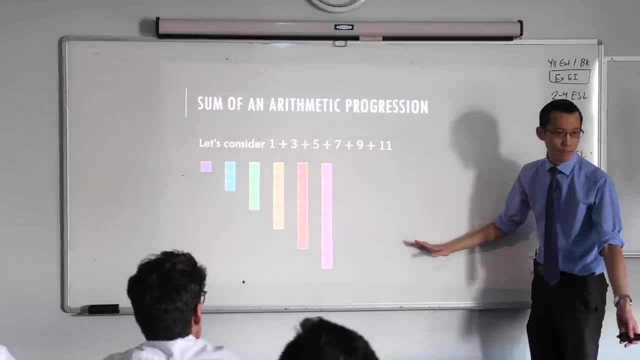 So here's the way I'm going to do it. Like I said before, I want to do this very visually. Do you agree that this is a way to represent 1 plus 3 plus 5 plus 7, etc. Are you happy with that? 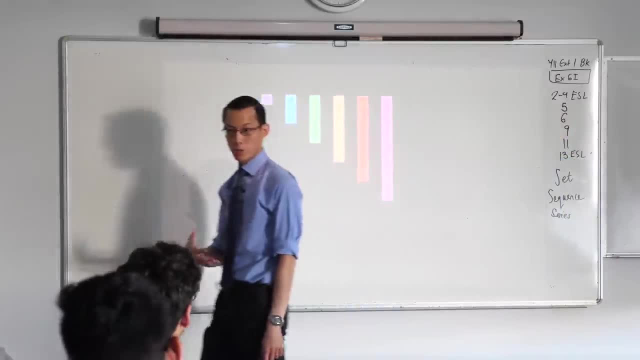 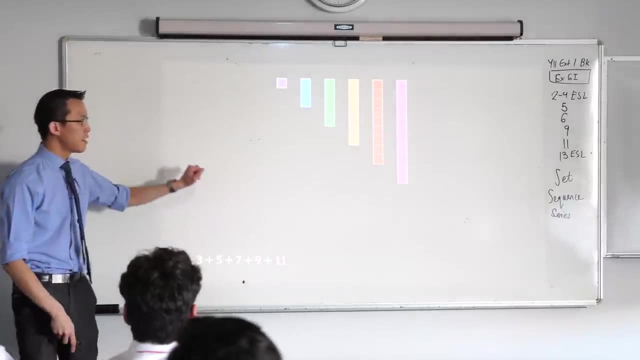 Okay, So what I want to do is have a little bit of a play with this visual representation. Okay, Now, for starters. this is what we've got: one all the odd numbers from 1 through to 11.. Okay, 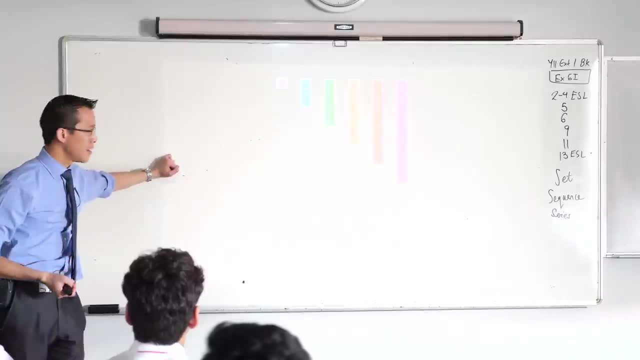 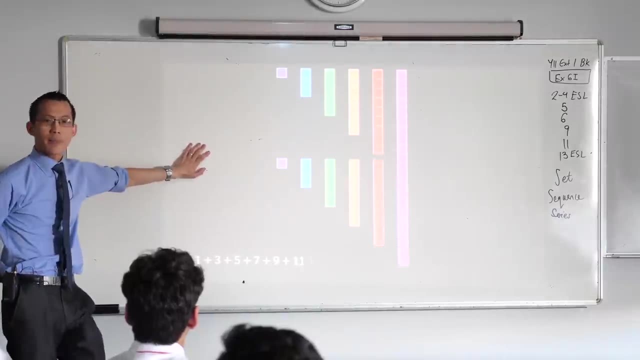 Now, what I'm going to do next is going to look like it makes things worse, but it actually takes advantage of a feature that an arithmetic progression has. Here's what I'm going to do: I'm going to make another copy of this arithmetic progression. 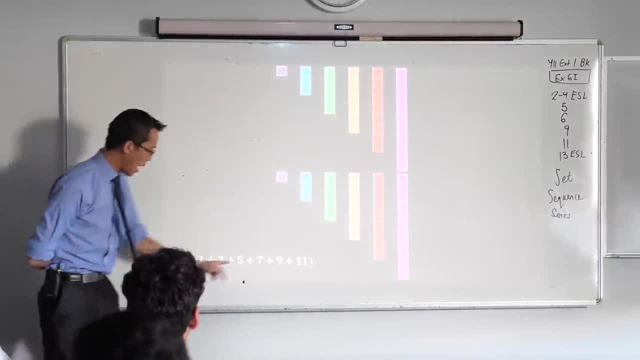 So I don't have 1 plus 3 plus all the way to 11.. I've got double that. Are you okay with that? so far Okay, And we still don't know what that's equal to, but that's okay. 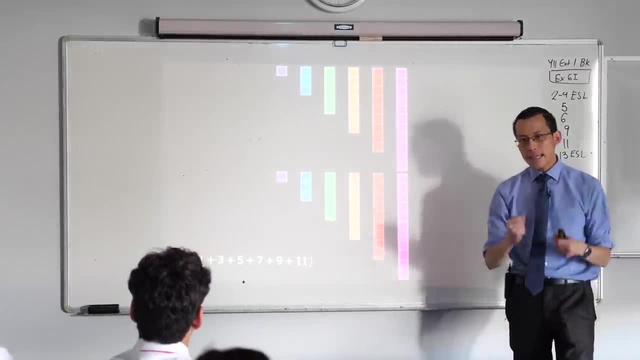 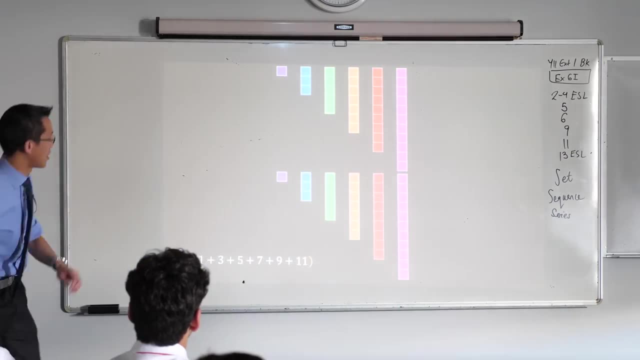 Now let me just wind back for a second to explain why I might do this. What is it that makes an arithmetic progression like this? What makes this an arithmetic progression as compared to say, for example, 1 plus 3 plus 5 plus 8?? 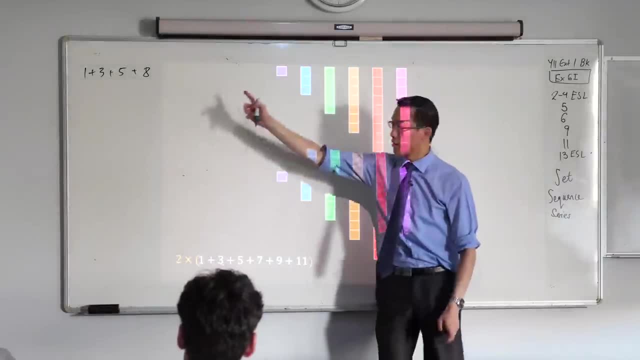 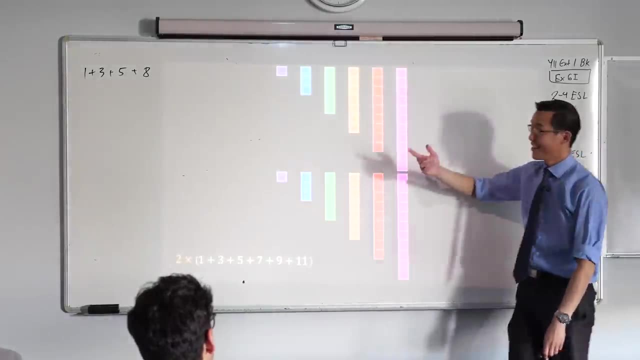 That is not an arithmetic progression. What does this have that that doesn't Go ahead. It's got a consistent pattern. Thank you, Tyler. It's consistent. in what way? How can you describe that pattern? It has a common difference. 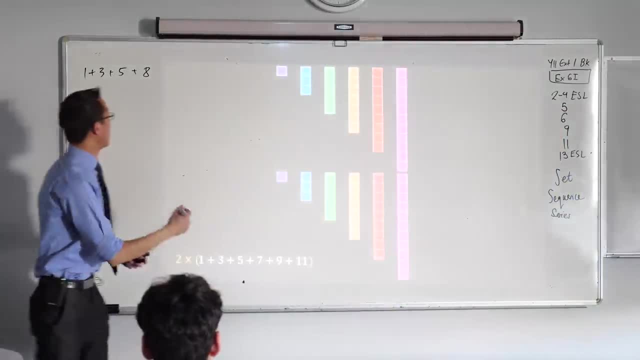 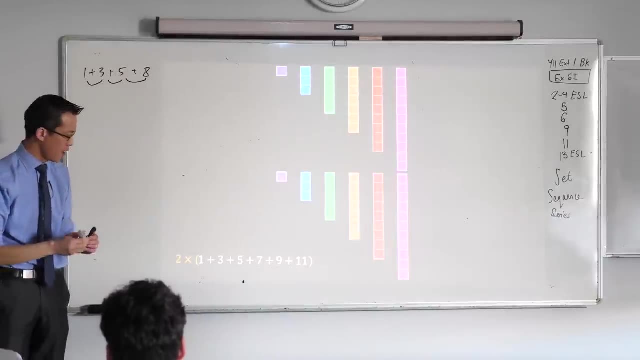 It's got a common difference, Thank you, That's the key, right? What we're looking for is: from here to here is 2.. From here to here is 2.. I'd like the next thing to also be the same difference, right. 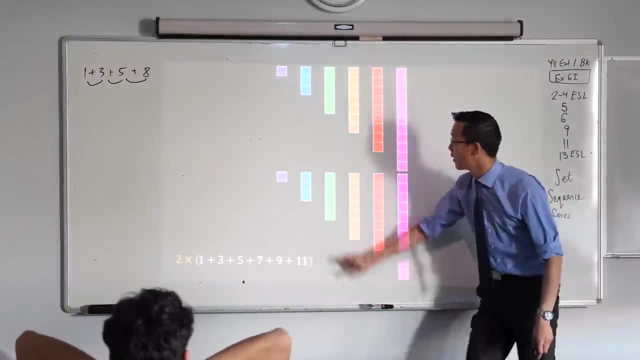 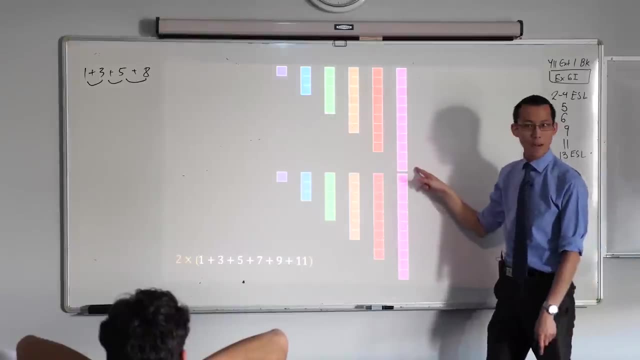 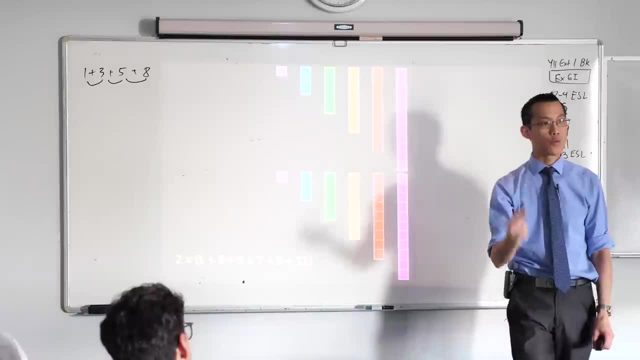 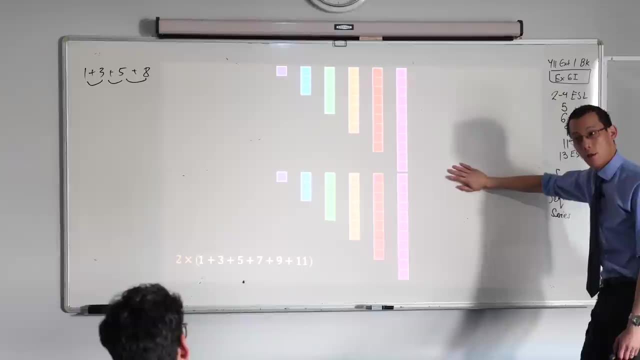 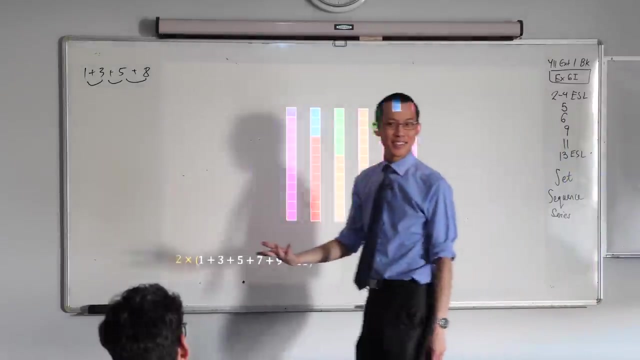 Like the difference is the same, going backwards. So watch really carefully, Because I've got two copies of this. now I can rearrange them in a way that's more helpful, namely like this: Now, why is this a more helpful way to think about it, right? 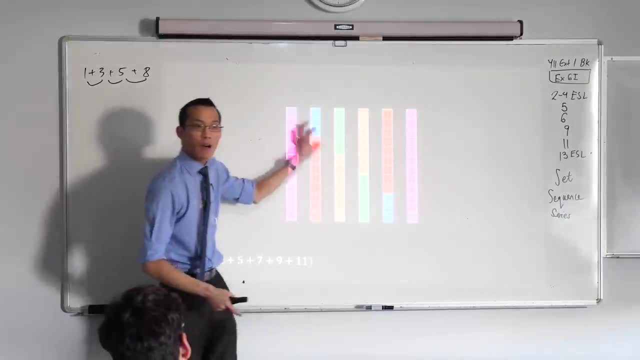 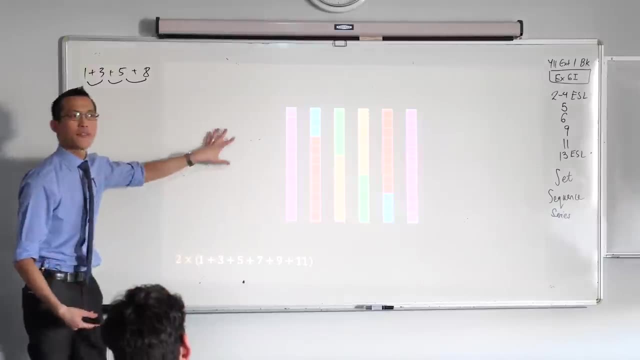 Well, number one, because it's arithmetic: how it grows is the same as how it shrinks. I'm just looking at it from two different perspectives. yeah, But secondly, the reason why this is so vastly superior is because I've got a rectangular array. 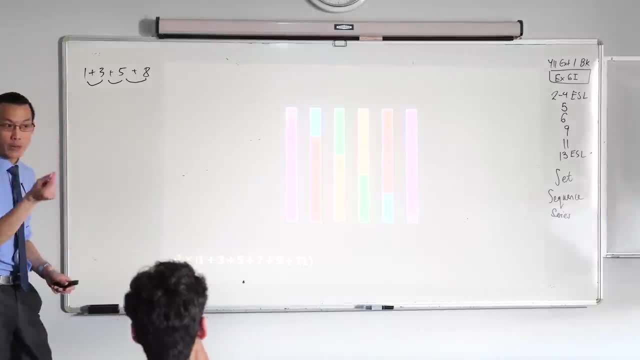 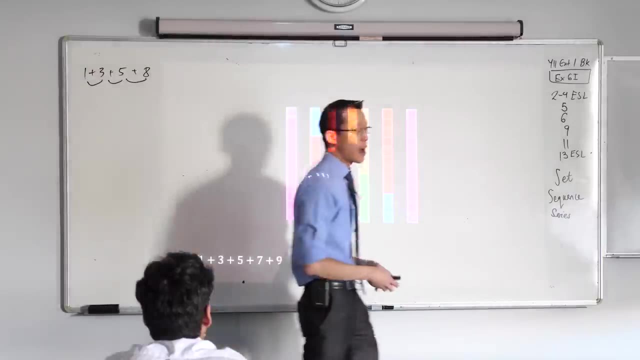 and we can work out the total size of this really, really quickly. Before we do that, I just want to highlight each of these columns that I've got. they're the same height. I could describe that height in a bunch of different ways. 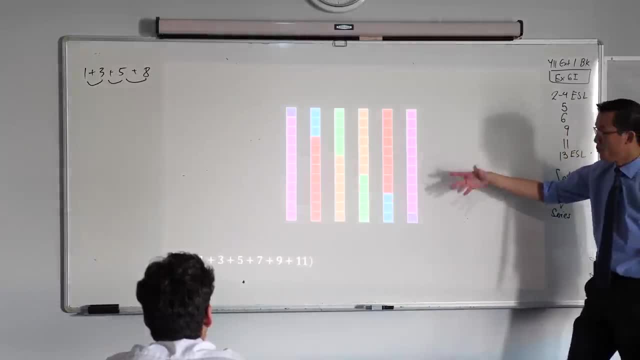 but again, look carefully, the change is subtle. A way that I think would be helpful is that each of these columns is the same as the first column, And the first column, of course, is made up of the first and the last term. 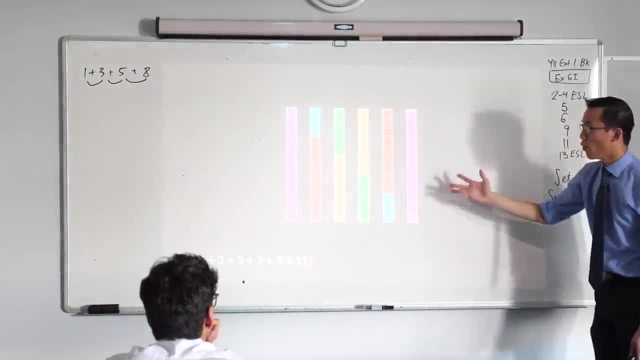 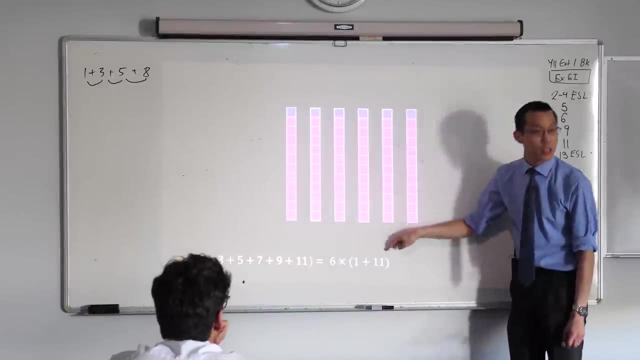 jammed together. Does that make sense? So if we consider them all as the same column, you can see I've got six lots, six columns, each of which is the first plus the last term. You with me. so far, Okay, so far, so good. 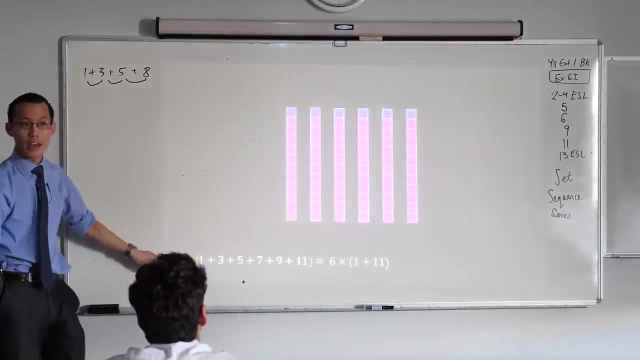 So, now that I've done the visual, I now want to think about this. This is what's going to help me, okay? So when we think about this, this is the part that I want. Actually, there's not much work that needs to be done. 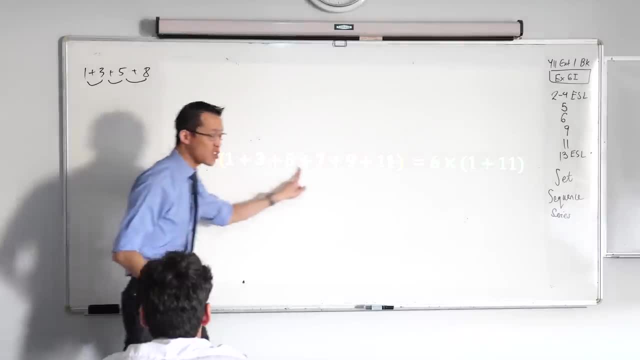 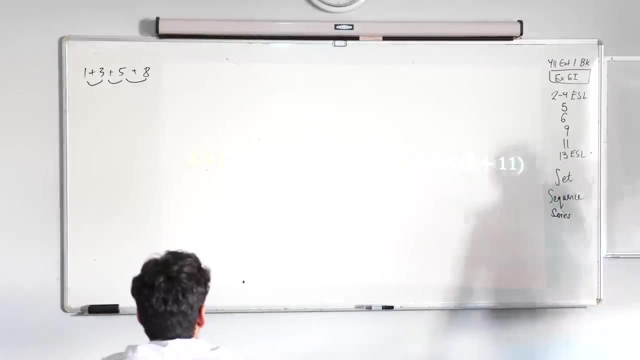 What operation do I need to conduct on both sides? that gives me just the original arithmetic series. What do I do to both sides? Let's get this. Hold that thought. get a student career. Who are you looking for, Aditya? 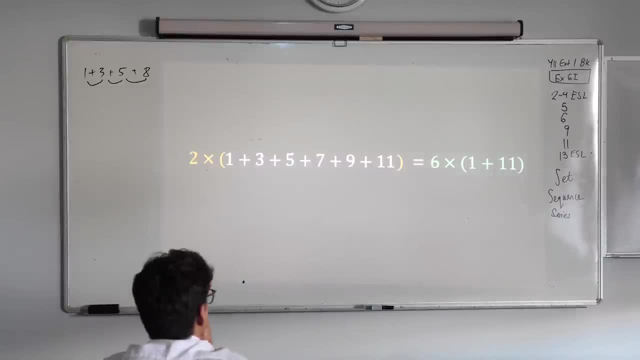 Lunchtime, He remembers. Thank you, Anyone else? Yeah, that's fine, 823.. 823.. You know the drill. Okay, I hit pause on you. Can you tell me What's the thing I do to both sides? 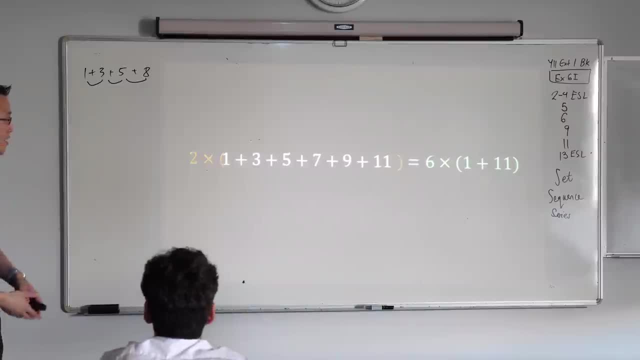 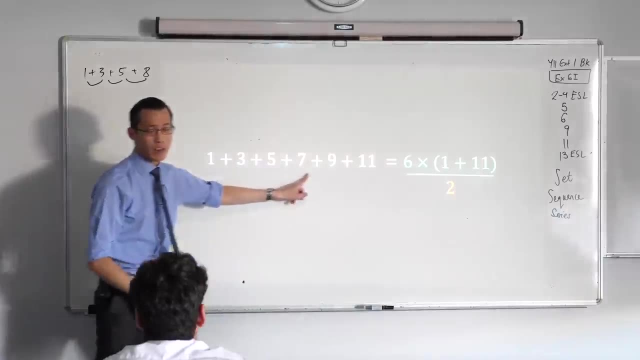 I divide by two, right, Okay, now this is what I want, But now that I've got this, this is the real key. okay, This is just for a particular progression that you could have just added up by hand. okay.